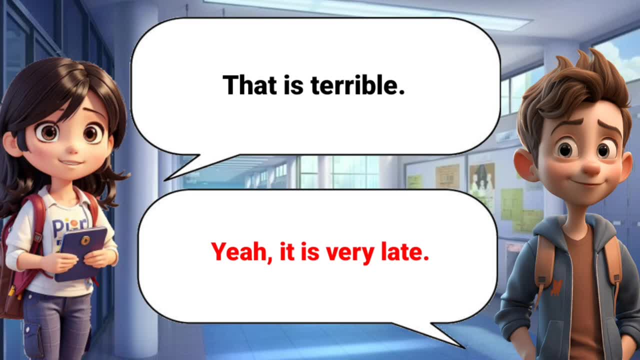 That is terrible. Nice to meet you. Bye, It is very late. Mine is next week. Why is your date so early? Mine is next week. Why is your date so early? I am a student athlete. Maybe I should play a sport. 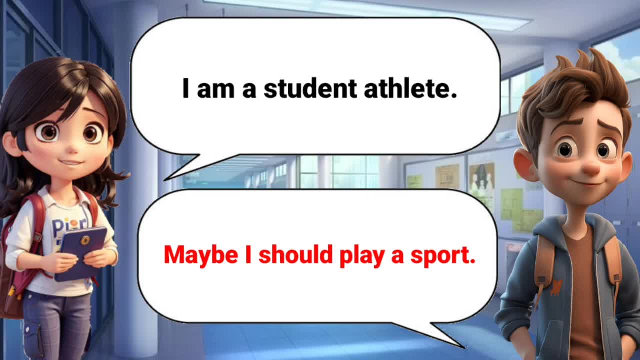 I am a student athlete. Maybe I should play a sport. Soccer tryouts are tomorrow. I don't like soccer. Soccer tryouts are tomorrow. I don't like soccer. Would you rather have a late registration date? I actually would. Would you rather have a late registration date? 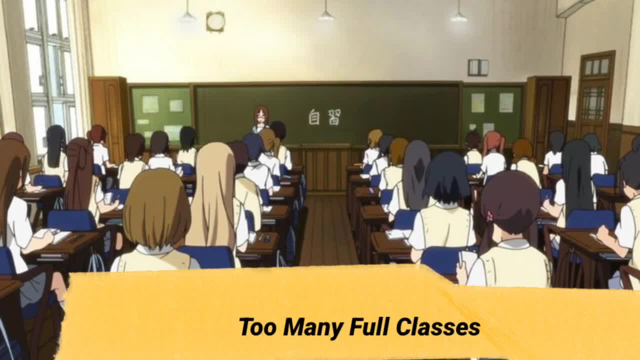 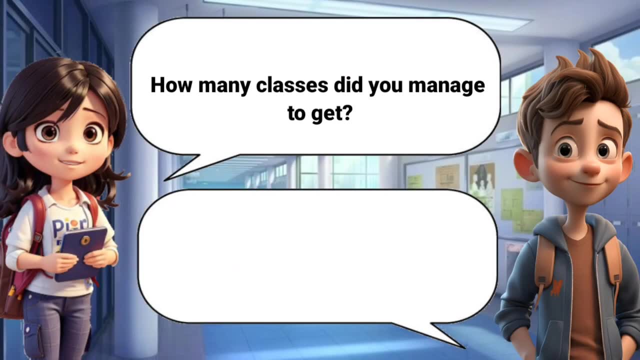 I actually would. Too many full classes. How many classes? How many classes did you manage to get? I only got two. How many classes did you manage to get? I only got two, I only got one. There are too many full classes at this college. 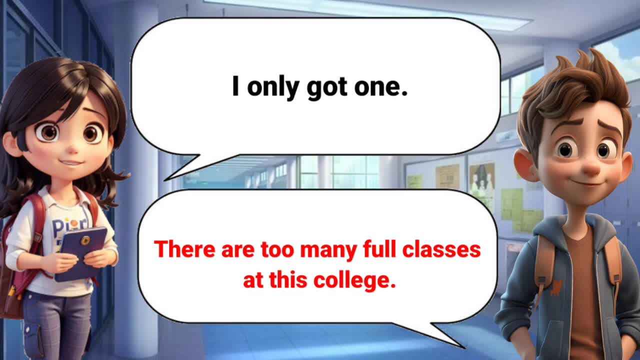 I only got one. There are too many full classes at this college. I never get the classes I need. Have you tried asking the professor for a spot? I never get the classes I need. Have you tried asking the professor for a spot? 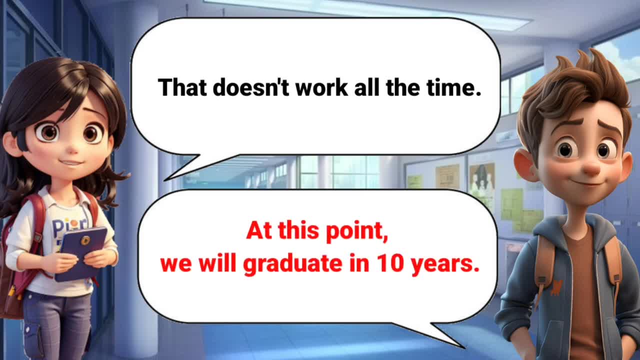 That doesn't work all the time. At this point. we will graduate in 10 years. That doesn't work all the time At this point. we will graduate in 10 years. That is so early. What are you talking about? 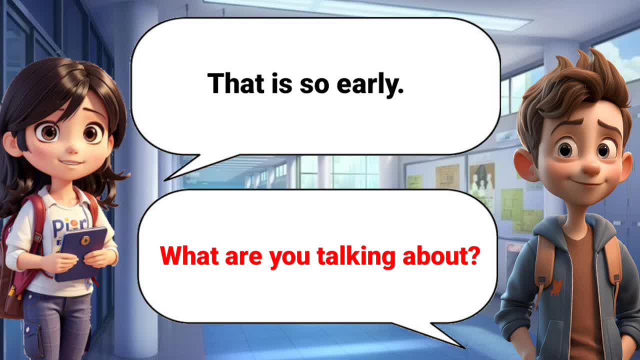 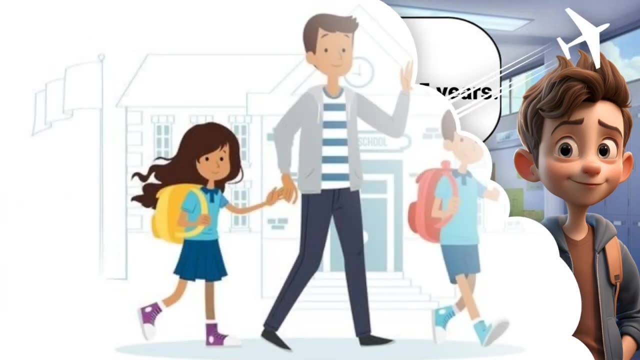 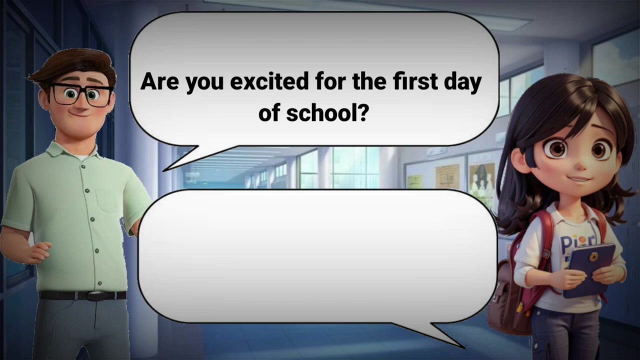 That is so early. What are you talking about? I think we will graduate in 15 years. You are funny. I think we will graduate in 15 years. You are funny. First day of school. Are you excited for the first day of school? 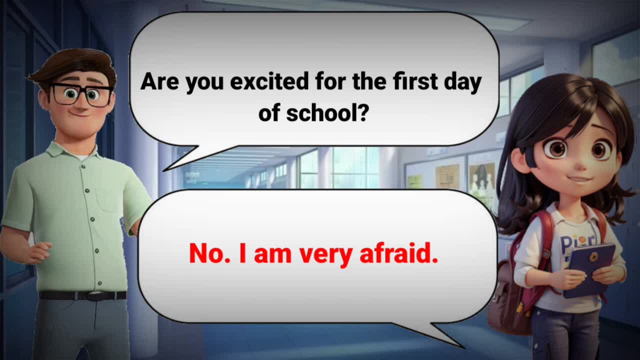 No, I am very afraid. Are you excited for the first day of school? No, I am very afraid. What is to be afraid about? I am afraid of the teacher. What is to be afraid about? I am afraid of the teacher. 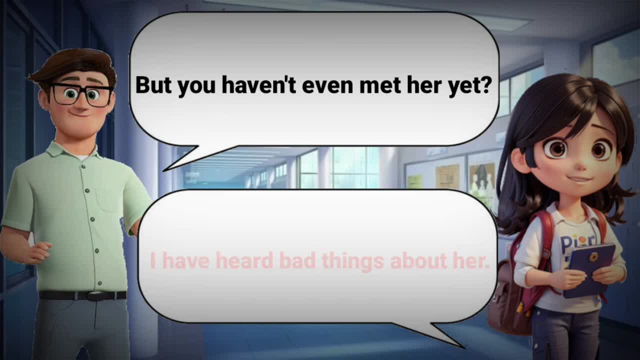 But you haven't even met her yet. I have heard bad things about her, But you haven't even met her yet. I have heard bad things about her. What bad things. I heard that she doesn't let anyone laugh. What bad things. 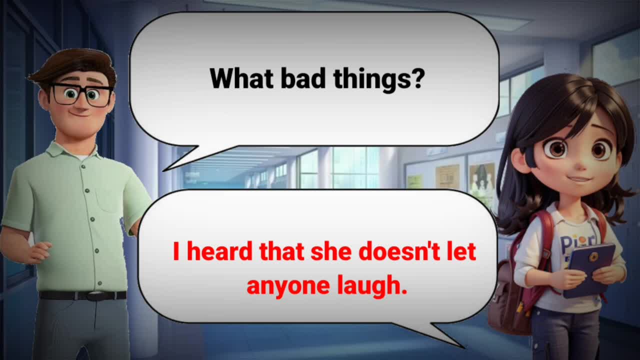 I heard that she doesn't let anyone laugh. That is ridiculous. The older kids told me that That is ridiculous. The older kids told me that They're just trying to scare you. Oh really, thank goodness They're just trying to scare you. 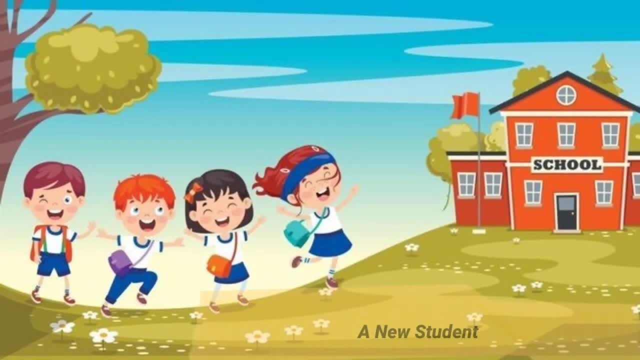 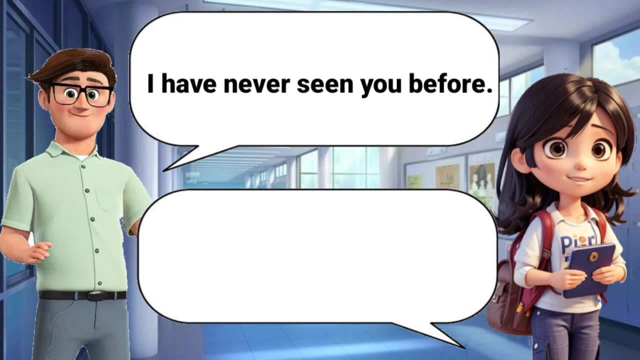 Oh really, thank goodness. A new student. I have never seen you before. I am a new student. I have never seen you before. I am a new student. Where are you from? I am from Japan. Where are you from? 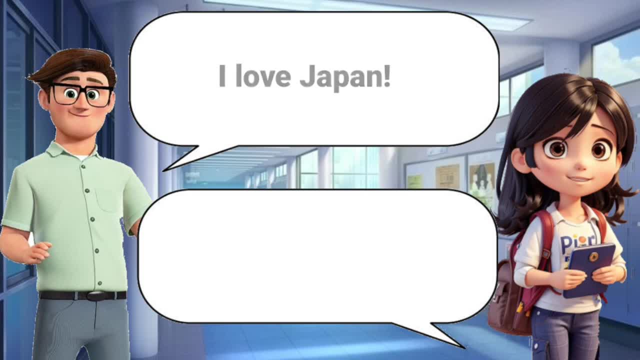 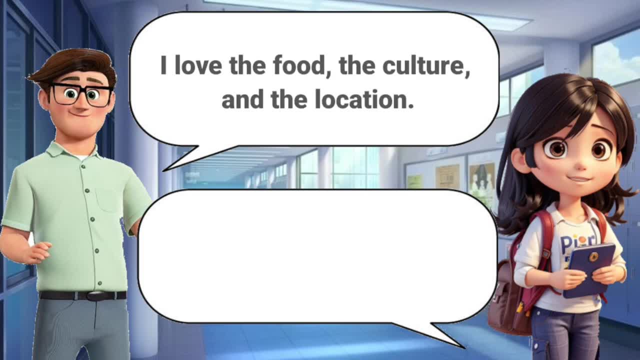 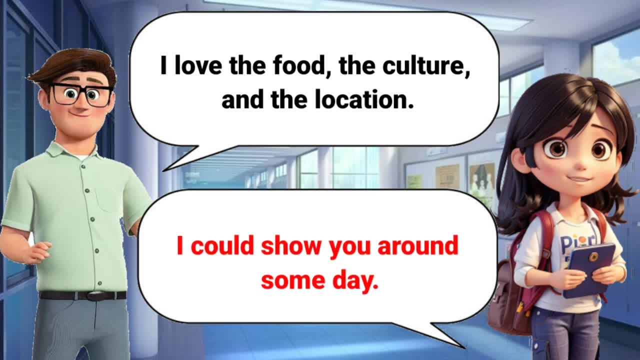 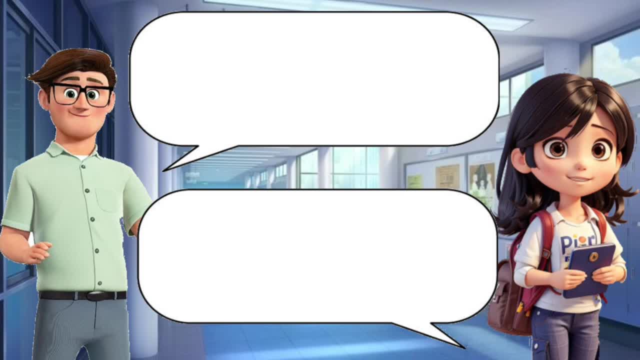 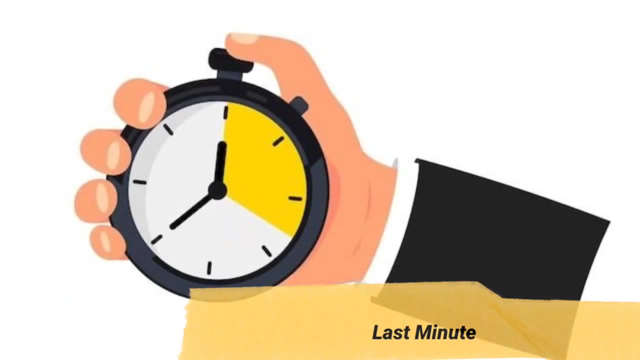 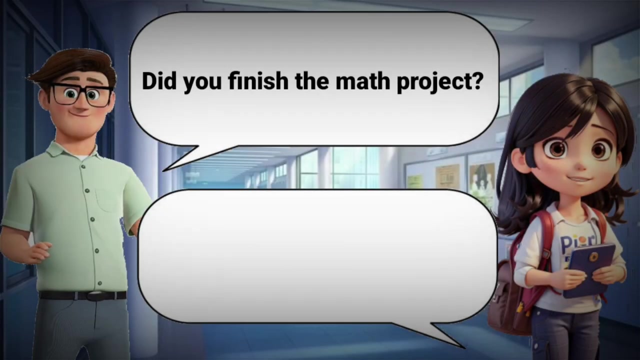 What do you love about Japan? What do you love about Japan? What do you love about Japan? That would be so fun. It would be my pleasure. Last minute Did you finish the math project? I have not started, But it's due tomorrow. 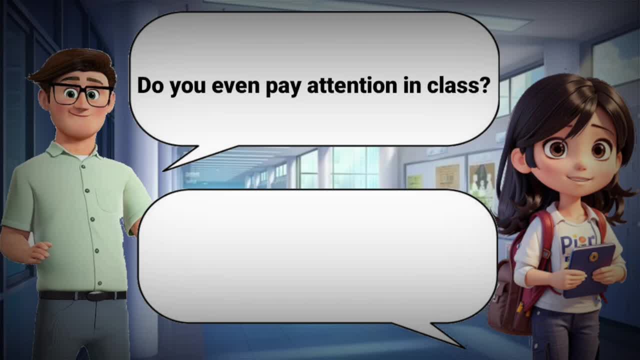 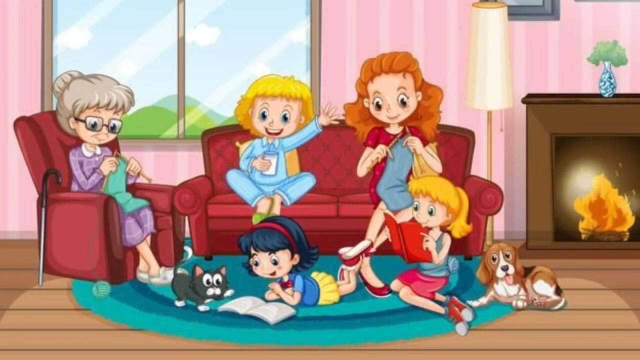 Do you even pay attention in class? I guess not. Do you know where to start? Not at all. I can help you. That would be awesome. I'll help you at my house tonight. I'll be there For getting it at home. 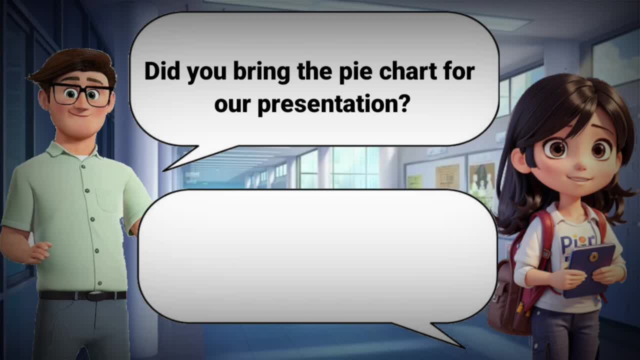 Did you bring the pie chart for our presentation? You're going to be mad. Did you bring the pie chart for our presentation? You're going to be mad. What did you do? I forgot the pie chart. What did you do? I forgot the pie chart. 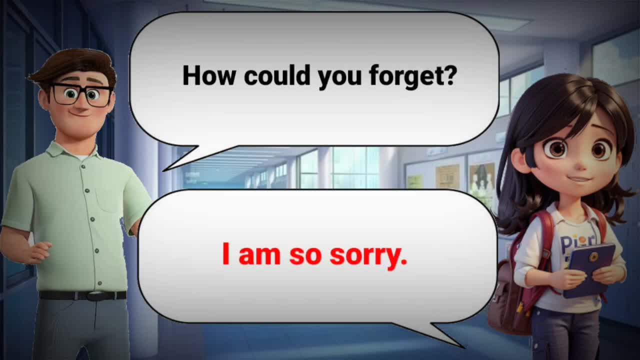 How could you forget? I am so sorry. How could you forget? I am so sorry. Where is it? It is at home. Where is it? It is at home? Are your parents at home? My mom is at home. Ask her to drop it off. 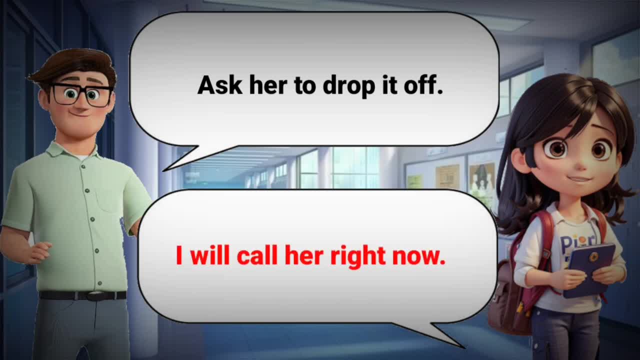 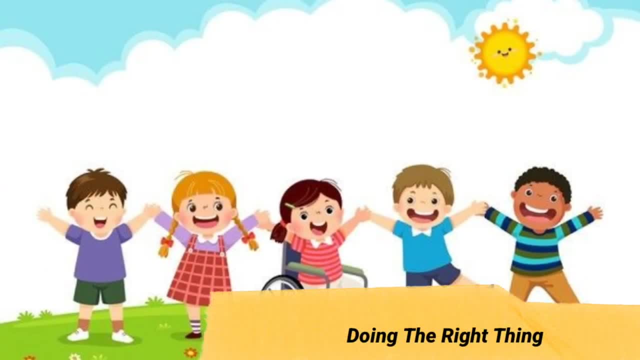 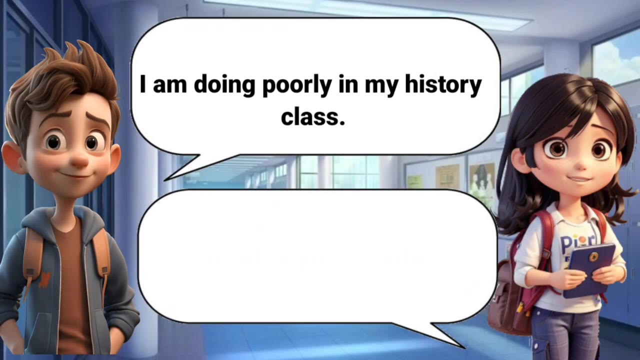 I will call her right now. Ask her to drop it off. I will call her right now. Doing the right thing. I am doing poorly in my history class. What is your grade? I am doing poorly in my history class. What is your grade? 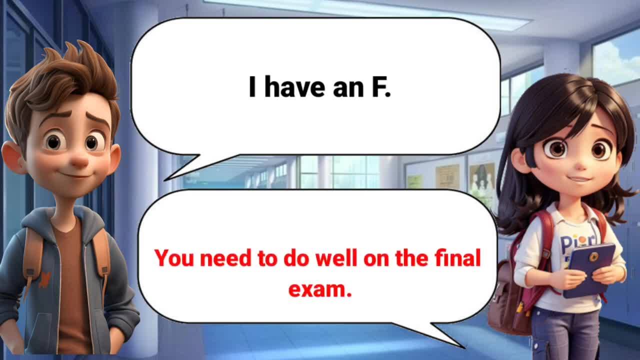 I have an F: You need to do well on the final exam. You need to do well on the final exam. I have an F: You need to do well on the final exam. I am planning to study. I am planning to study. 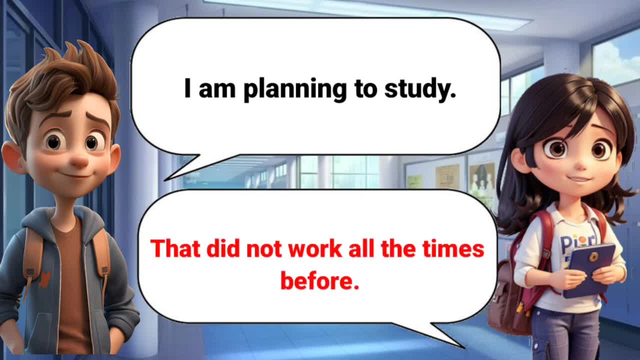 That did not work all the time before. That did not work all the time before I am planning to study. That did not work all the time before. That did not work all the time before. What do you think I should do then? 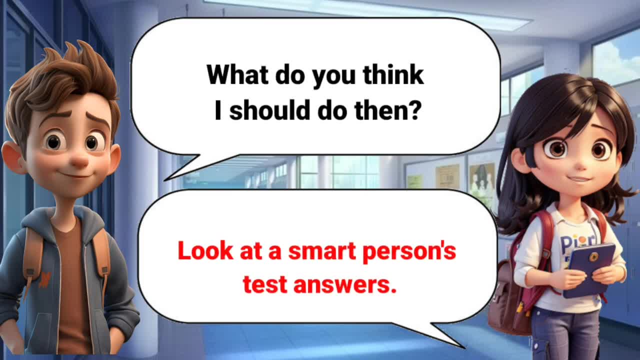 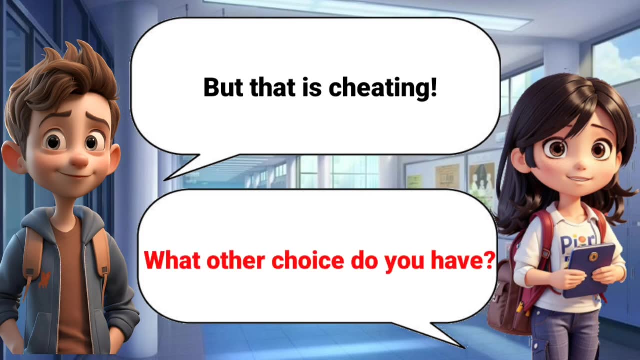 What do you think I should do then? Look at a smart person's test answers. Look at a smart person's test answers. What do you think I should do then? Look at a smart person's test answers. But that is cheating. What other choice do you have? 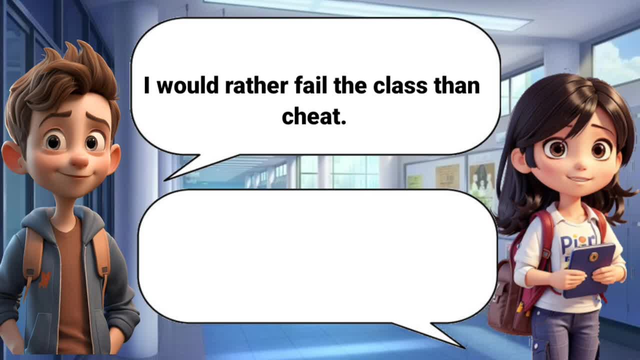 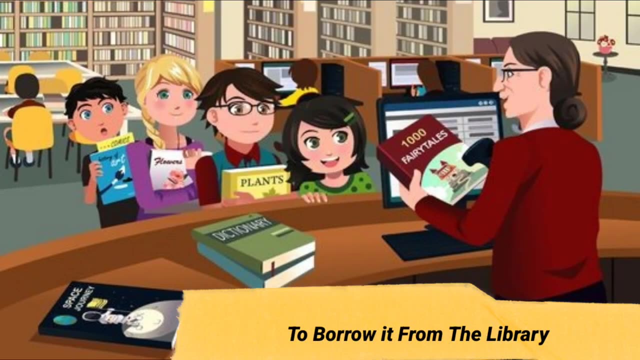 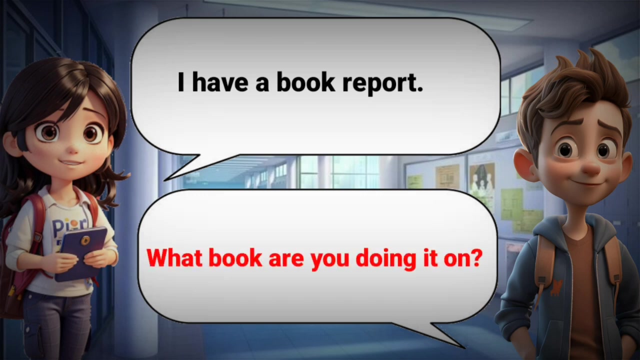 I would rather fail the class than cheat. You're a good student. I would rather fail the class than cheat, You're a good student. To borrow it from the library: I have a book report. What book are you doing it on? 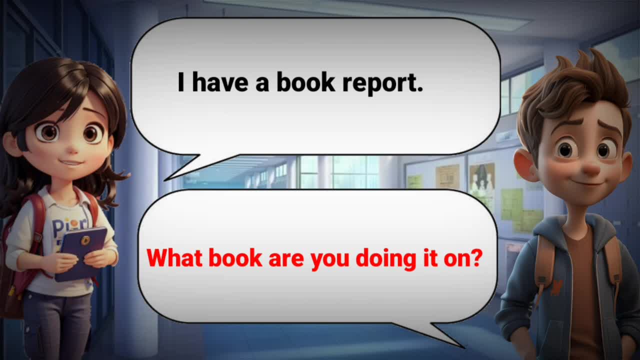 I have a book report. What book are you doing it on? I have to read To Kill a Mockingbird. That is an excellent book. I have to read To Kill a Mockingbird. I have to read To Kill a Mockingbird. 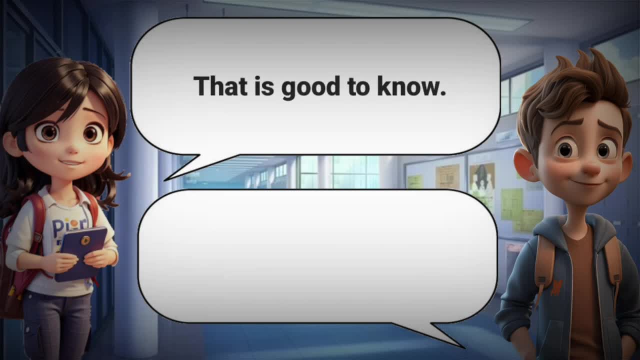 That is an excellent book. That is good to know. Do you have the book yet? That is good to know. Do you have the book yet? I am planning to get it soon. You should borrow it from the library. I am planning to get it soon. 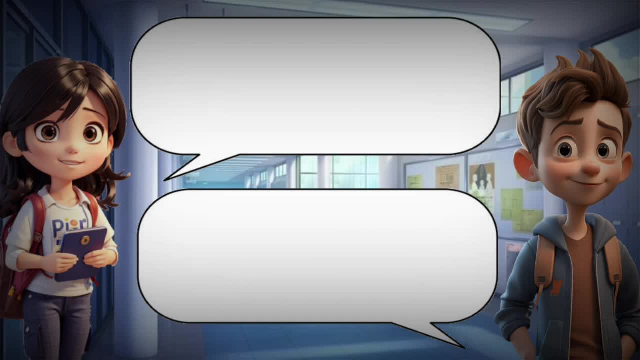 You should borrow it from the library. You should borrow it from the library. What is the library? You have never heard of the library. You have never heard of the library. What is the library? You have never heard of the library. You have never heard of the library. 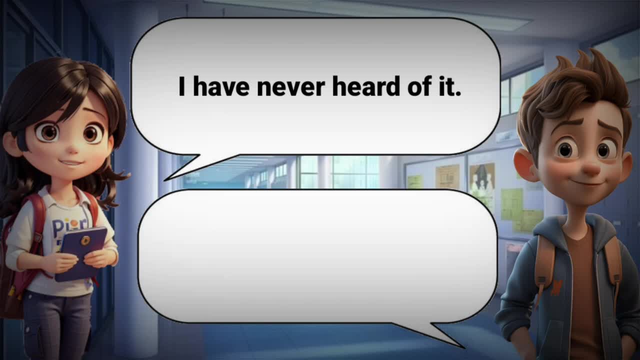 I have never heard of it. I have never heard of it. At the library, you can borrow books for free. At the library, you can borrow books for free. I have never heard of it. I have never heard of it. At the library, you can borrow books for free. 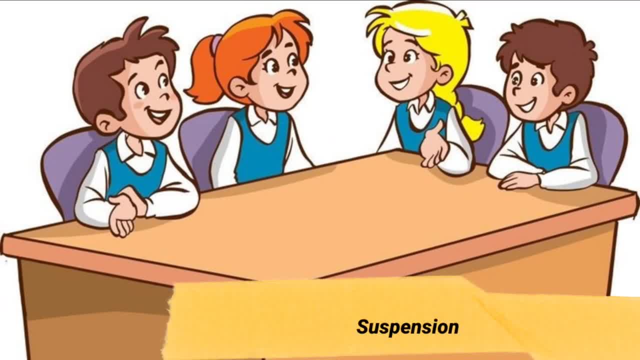 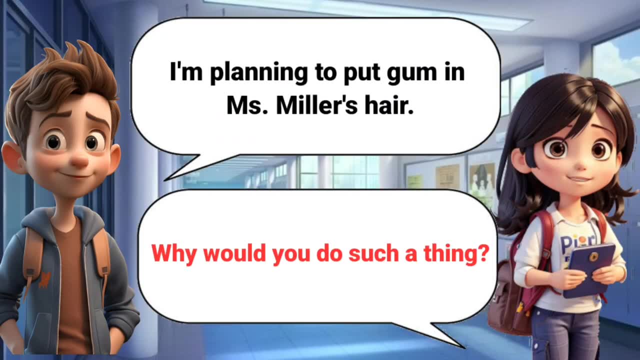 At the library, you can borrow books for free. I'm planning to put gum in Ms Miller's hair. Why would you do such a thing? Because Ms Miller gives too much homework. She is so nice though, I do not care. 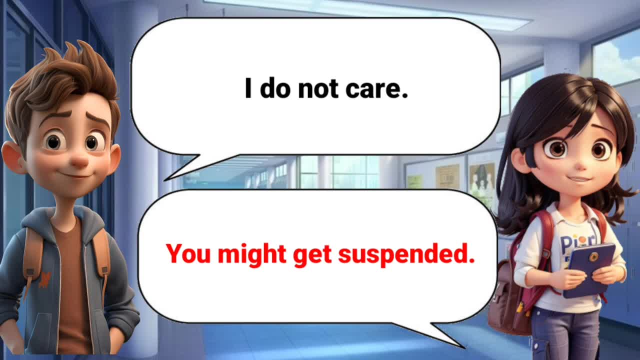 You might get suspended. What does that mean? It means you have to leave school for a while. That's the punishment. Yes, it is worse than detention. Suspension sounds like a vacation to me. Say that to your parents. Suspension sounds like a vacation to me. 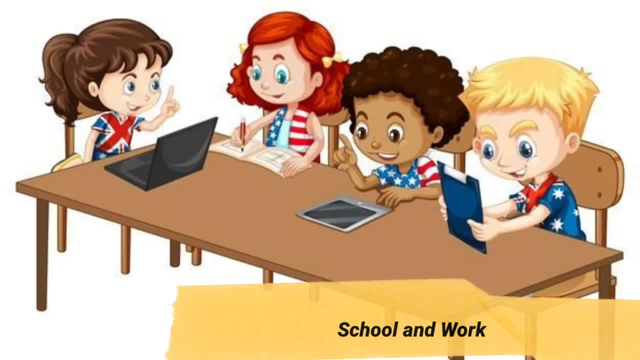 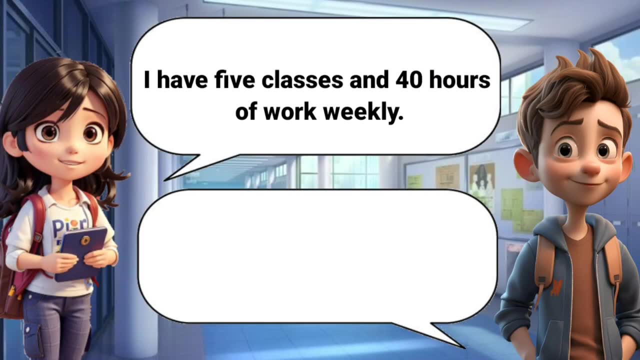 Say that to your parents. School and work: I have 5 classes and 40 hours of work weekly. Your life is so stressful. I have 5 classes and 40 hours of work weekly. Your life is so stressful. Sadly it is. 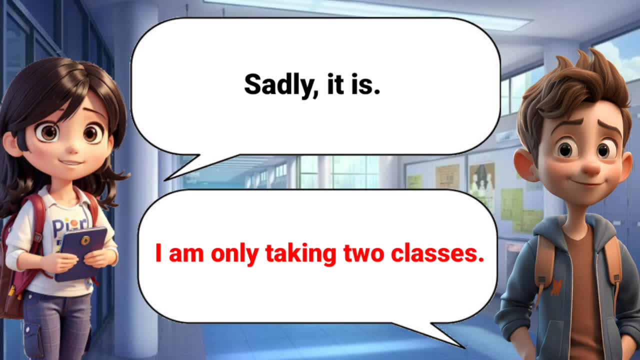 I am only taking 2 classes. Sadly it is. I am only taking 2 classes. Do you have work? I am too lazy to work. Do you have work? I am too lazy to work. Don't you want money though? 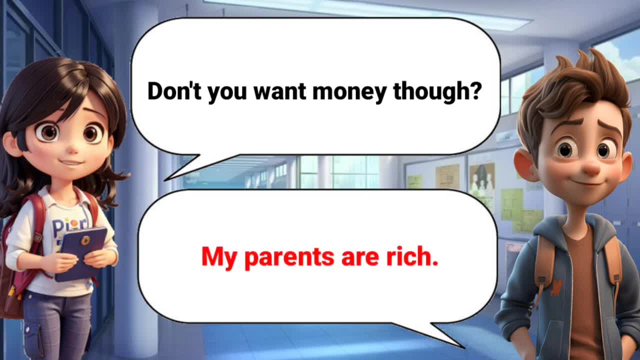 My parents are rich. Don't you want money, though? My parents are rich. My parents are poor. I'm sorry to hear that My parents are poor. I'm sorry to hear that They're poor, but honest, good people. Good for you. 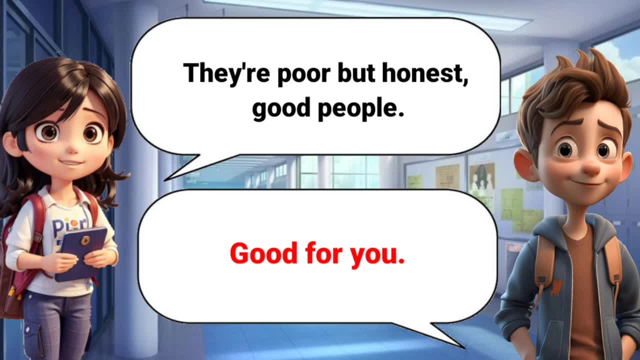 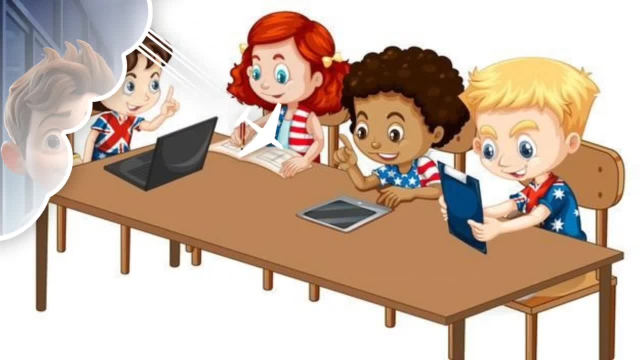 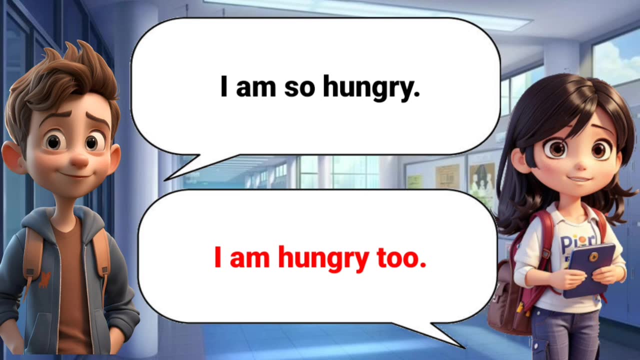 They're poor but honest, good people. Good for you. Eating in class. I am so hungry, I am hungry too. I am so hungry, I am hungry too. How many more minutes until lunch? 30 more minutes. How many more minutes until lunch? 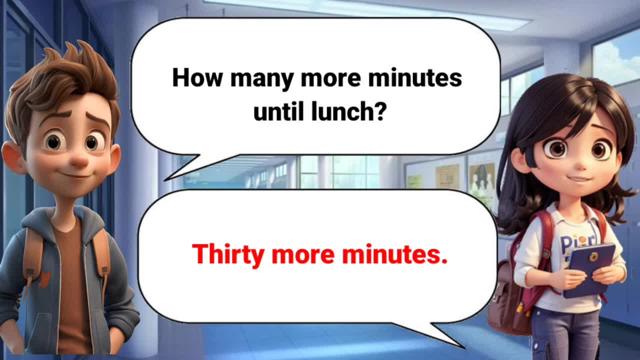 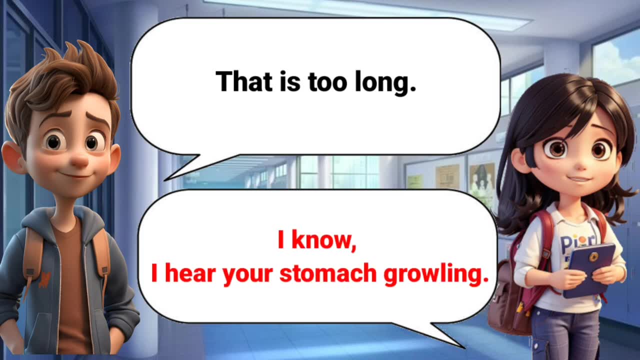 How many more minutes until lunch? 30 more minutes, That is too long. I know I hear your stomach growling. I know I hear your stomach growling. That is too long. I know I hear your stomach growling. 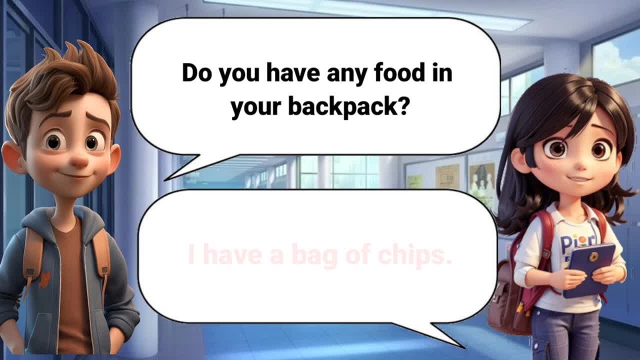 Do you have any food in your backpack? I have a bag of chips. Do you have any food in your backpack? I have a bag of chips. I have a bag of chips. Can I have some? Maybe next time Can I have some. 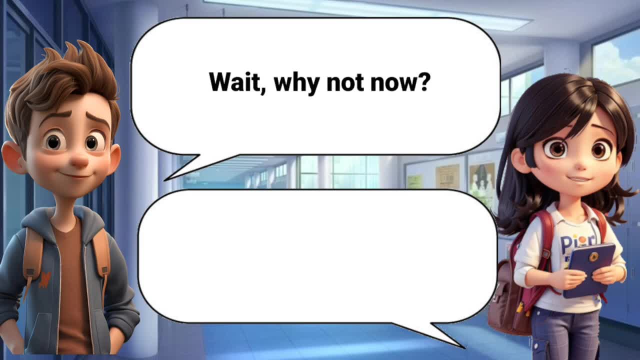 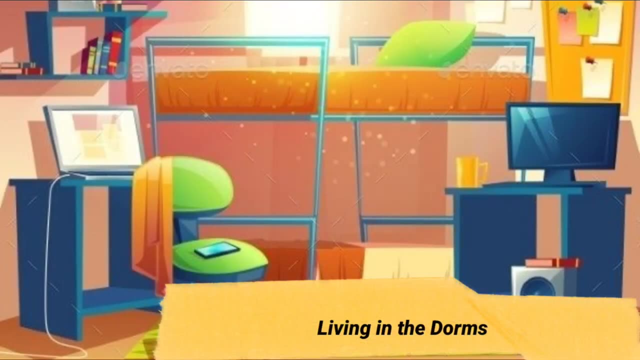 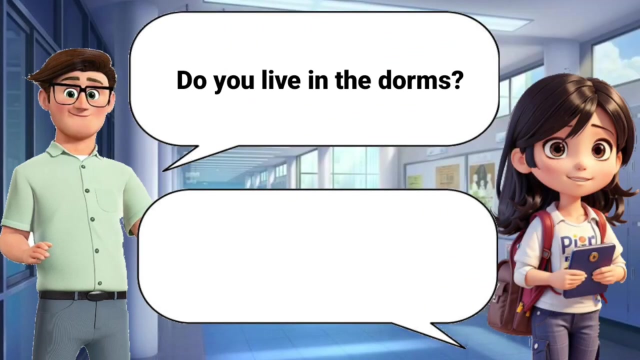 Maybe next time. Wait, why not now? Because I'm going to eat the chips. Wait, why not now? Because I'm going to eat the chips. Living in the dorms- Living in the dorms? Do you live in the dorms? 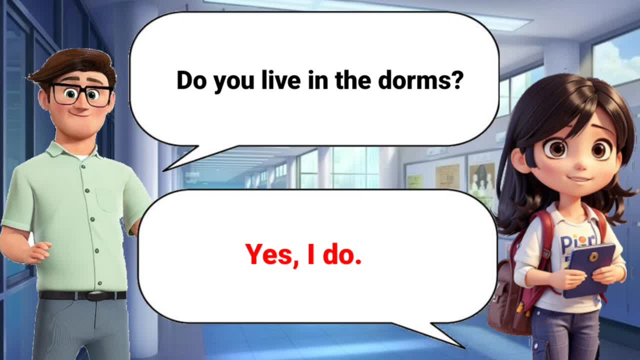 Yes, I do. Do you live in the dorms? Yes, I do. What do you like about it? I get to see my friends almost all the time. What do you like about it? I get to see my friends almost all the time. 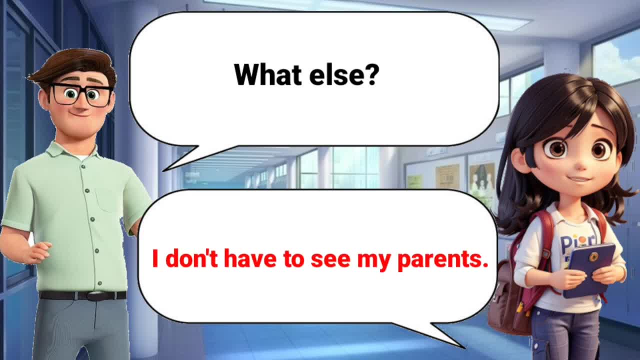 What else I don't have to see my parents? What else I don't have to see my parents? I don't have to see my parents? How much does it cost to dorm? It is very expensive. How much does it cost to dorm? 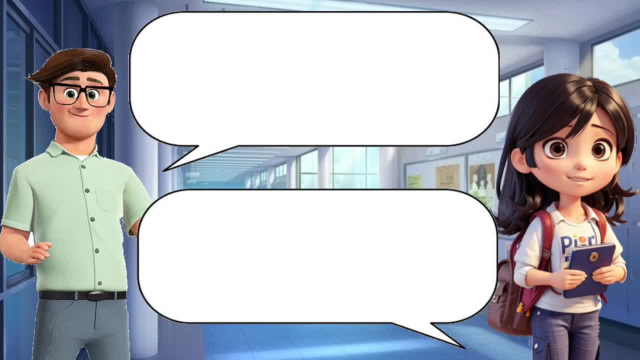 It is very expensive. Tell me exactly how much. Tell me exactly how much You're going to faint after I tell you. Tell me exactly how much You're going to faint after I tell you. Just tell me. It costs $15,000 per year. Just tell me It costs $15,000 per year. Popularity- I wish I was a cheerleader. Why do you want to be one? I wish I was a cheerleader. Why do you want to be one? Cheerleaders are popular. 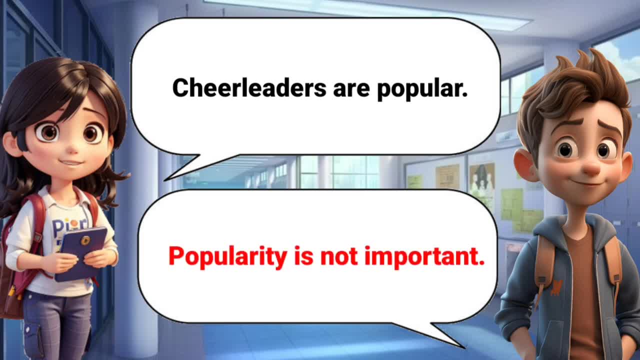 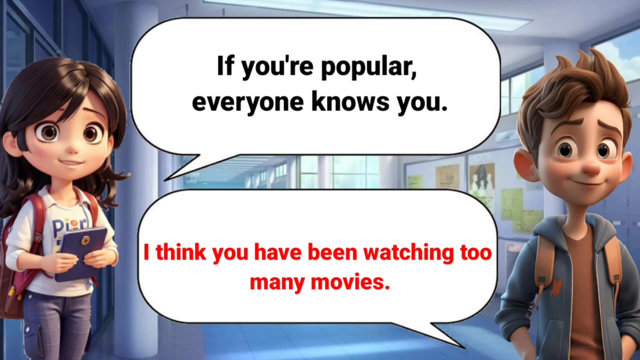 Popularity is not important. Cheerleaders are popular. Popularity is not important. If you're popular, everyone knows you. I think you have been watching too many movies. If you're popular, everyone knows you. I think you have been watching too many movies. 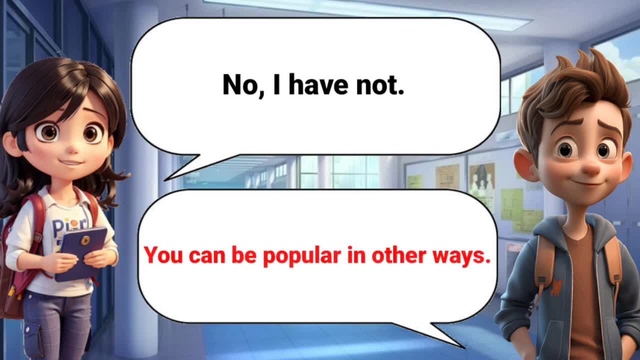 No, I have not, You can be popular in other ways. No, I have not, You can be popular in other ways. What other ways You could just say be nice to people? what other ways you could just be nice to people? 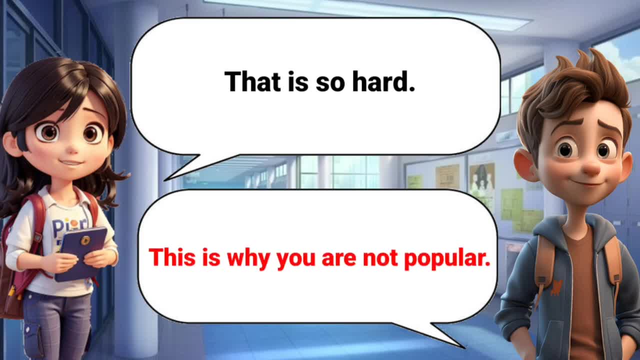 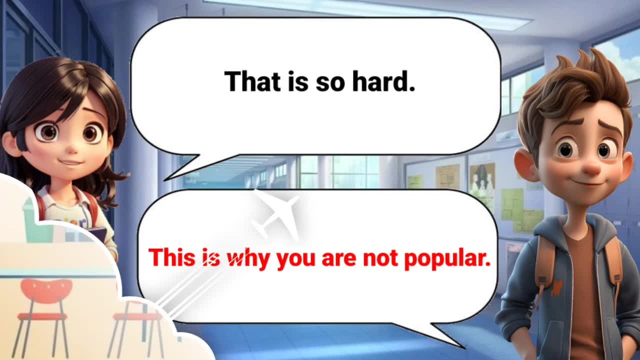 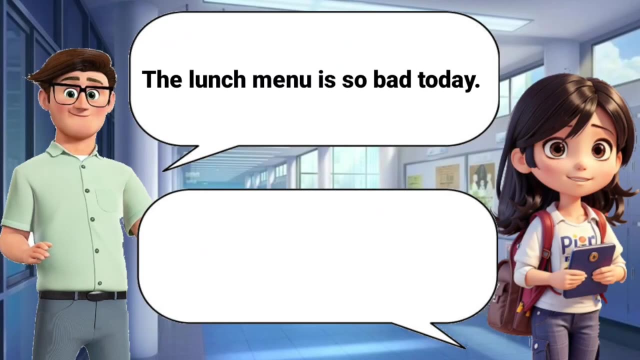 that is so hard. this is why you are not popular. that is so hard. this is why you are not popular. the vending machine- the lunch menu- is so bad today. what is the cafeteria serving? the lunch menu is so bad today. what is the cafeteria serving leftover meatloaf and brussels sprouts? that is disgusting. 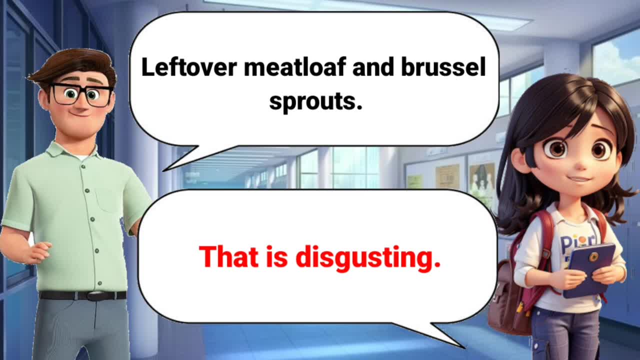 leftover meatloaf and brussels sprouts. that is disgusting. i'm thinking of buying something to eat. i'm thinking of buying something to eat from the vending machine- from the vending machine. i wouldn't do that if i were you. i wouldn't do that if i were you. i'm thinking of buying something from the 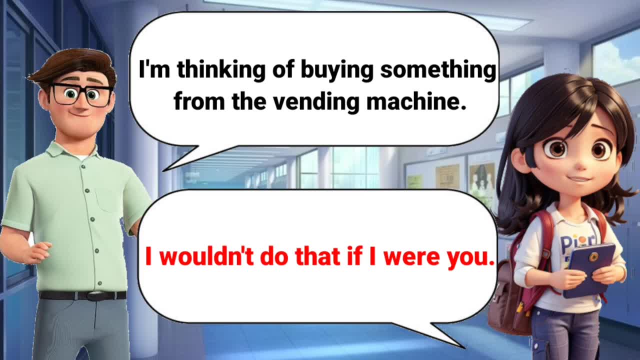 i'm thinking of buying something from the vending machine. vending machine. i wouldn't do that if i were you. what's wrong with the vending machine? it steals your money. it steals your money. what's wrong with the vending machine? what's wrong with the vending machine? it steals your money. 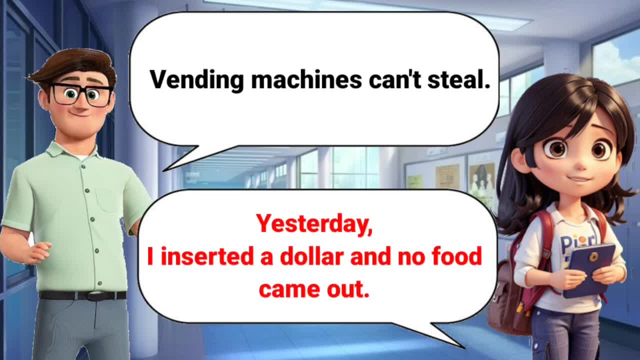 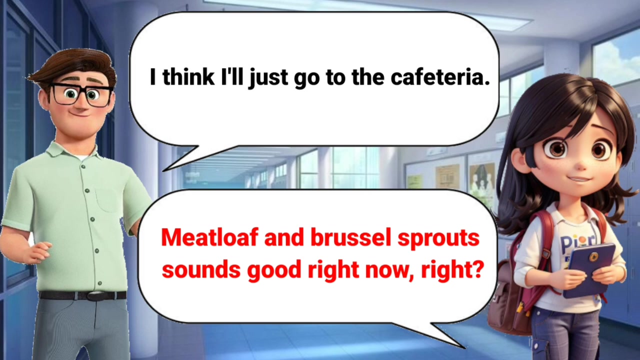 vending machines can't steal. Yesterday I inserted a dollar and no food came out. Vending machines can't steal. Yesterday, I inserted a dollar and no food came out. I think I'll just go to the cafeteria. Meatloaf and Brussels sprouts sounds good. right now, right. 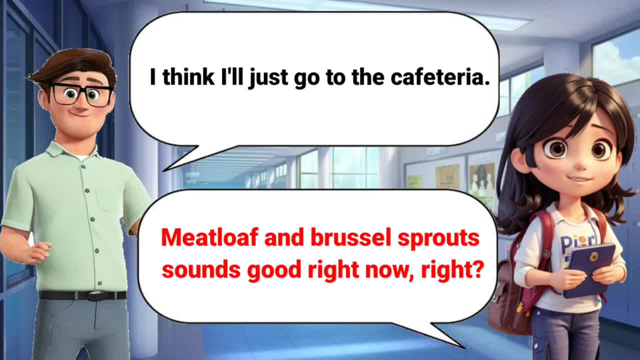 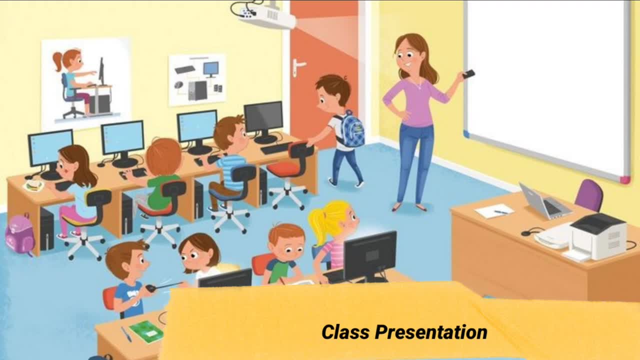 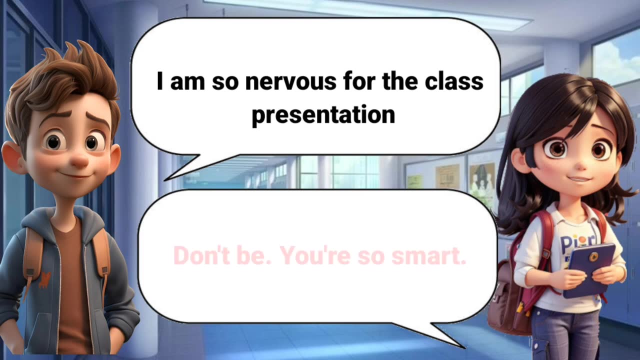 I think I'll just go to the cafeteria. Meatloaf and Brussels sprouts sounds good right now. right, Class presentation. I am so nervous for the class presentation. Don't be, you're so smart. I am so nervous for the class presentation. 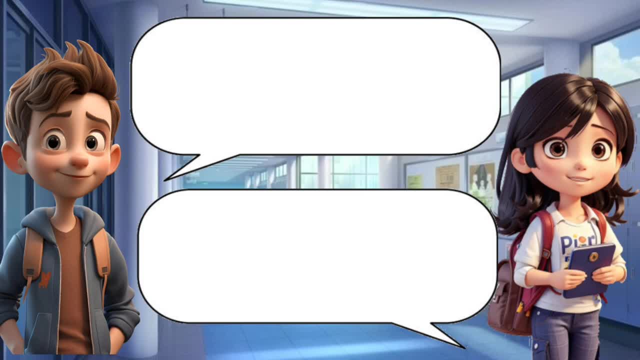 Don't be. you're so smart, I know, but I don't like a big audience. Do you want my advice? I know, but I don't like a big audience. Do you want my advice? Of course I do. 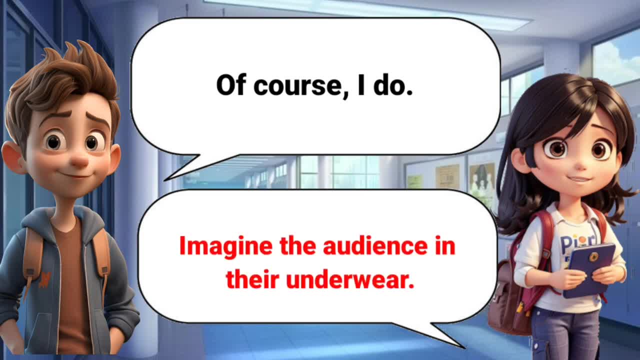 Imagine the audience in their underwear. Of course, I do Imagine the audience in their underwear. That is insane, It really works. That is insane, It really works. Have you tried it? Yes, I got an A on my presentation. 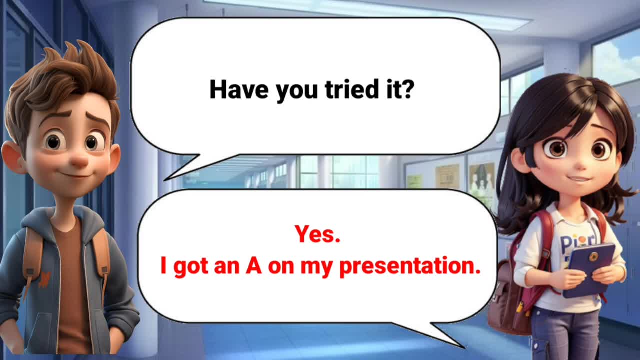 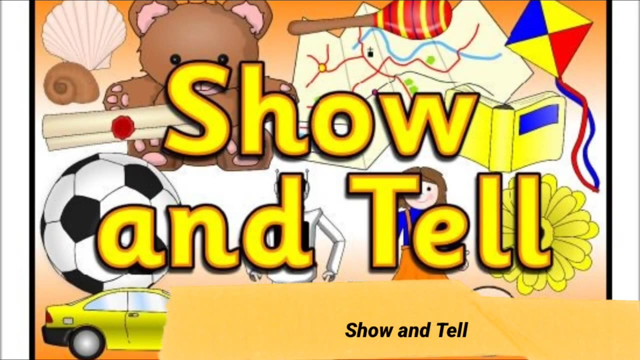 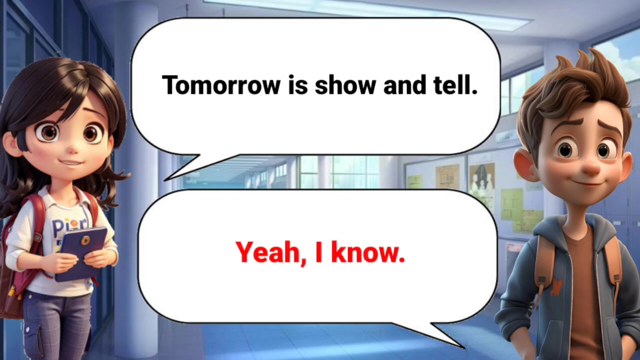 Have you tried it? Yes, I got an A on my presentation. I'll try it, then You can do it. I'll try it, then You can do it. Show and tell. Tomorrow is show and tell. Yeah, I know. 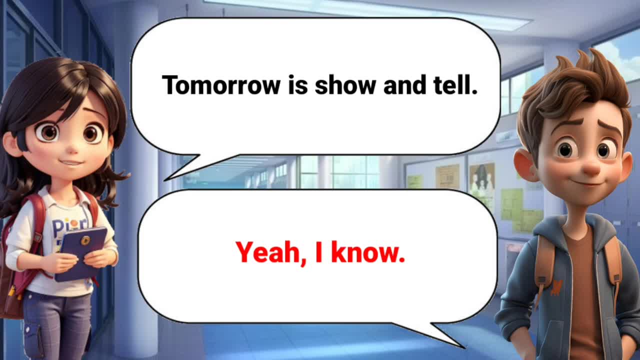 Tomorrow is show and tell. Yeah, I know, I am bringing my new purse for show and tell Purses are boring. I am bringing my new purse for show and tell. Purses are boring. No, they're not. Well, I'm bringing my dog. 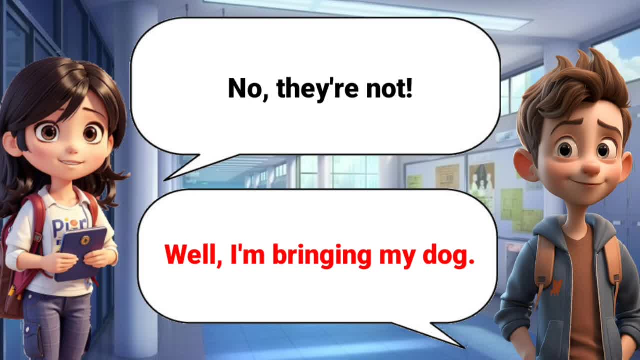 No, they're not. Well, I'm bringing my dog. You can't bring dogs to school. No one has to know until tomorrow. You can't bring dogs to school. No one has to know until tomorrow. You are going to get into so much trouble, But I'll be the coolest kid in school. 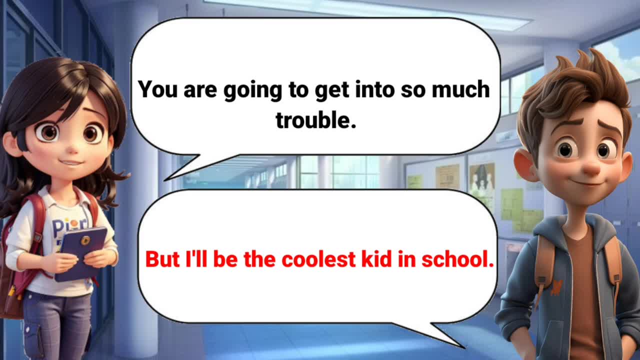 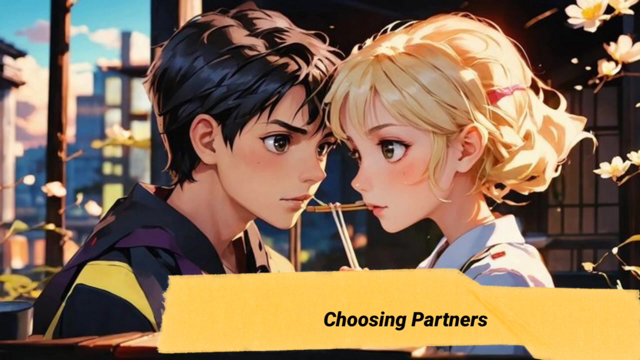 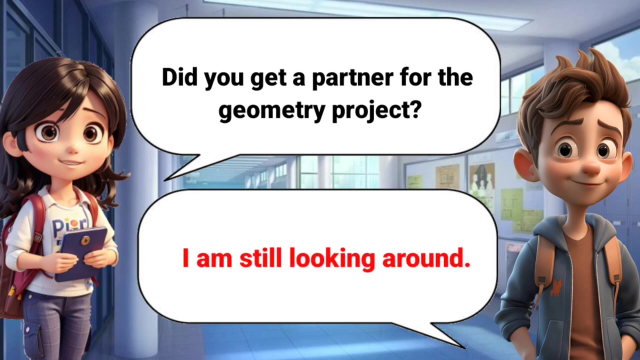 You won't be saying that in jail. I am not falling for that. You won't be saying that in jail, I am not falling for that. Choosing partners: Did you get a partner for the geometry project? I am still looking around. Did you get a partner for the geometry project? 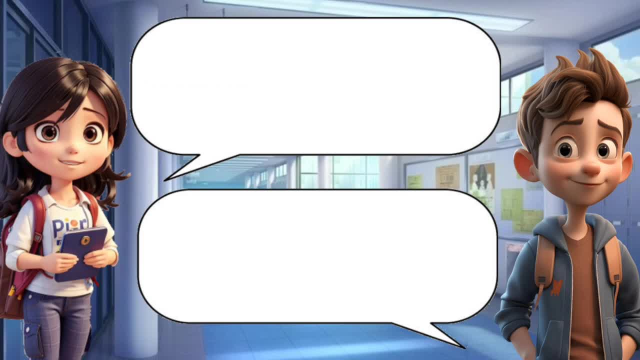 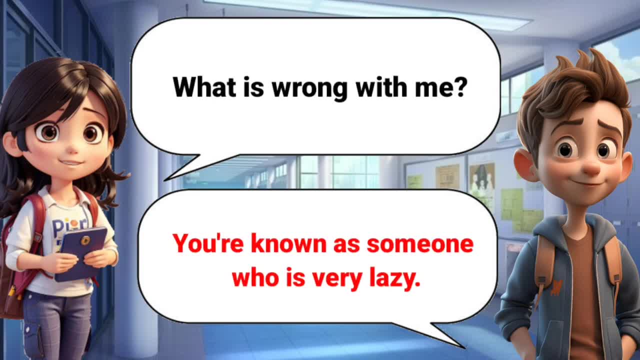 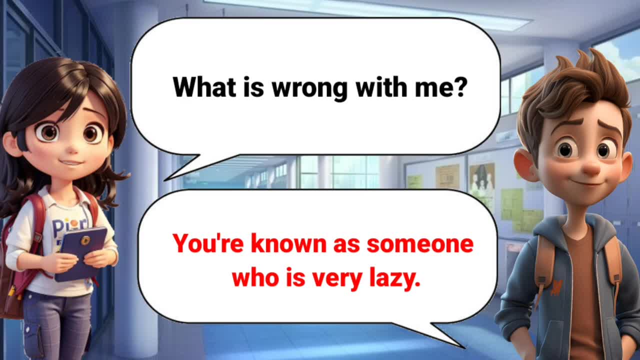 What is wrong with me? You're known as someone who is very lazy. That is so not true. Well, it's what I heard from our classmates. That is so not true. Well, it's what I heard from our classmates. You can't always trust people. 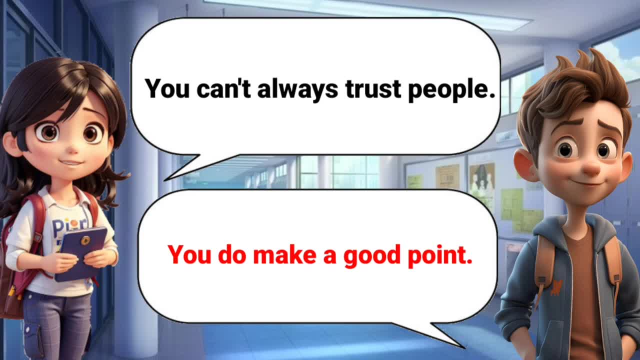 You do make a good point. You can't always trust people. You do make a good point. Give me a chance and I won't let you down. Okay, I trust you. Give me a chance and I won't let you down. 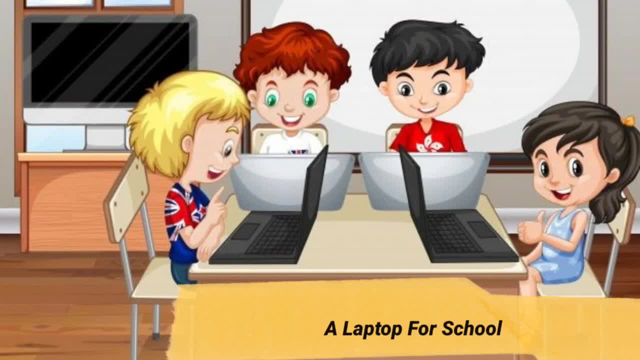 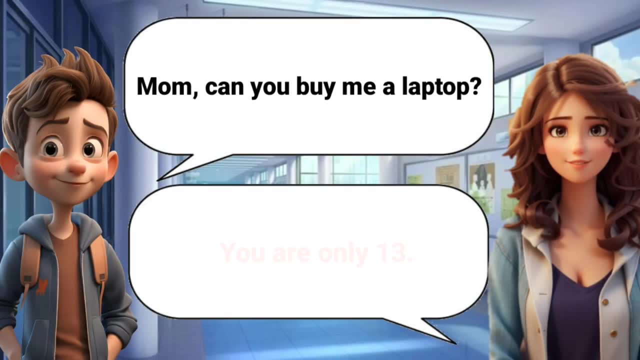 Okay, I trust you A laptop for school. Mom, can you buy me a laptop? You are only thirteen. Mom, can you buy me a laptop? You are only thirteen. Everyone in school has one. They must be rich then. 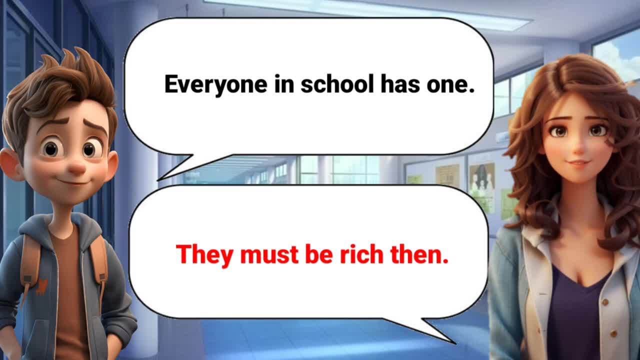 Everyone in school has one. They must be rich, then. I really need it. What do you need it for? I really need it. What do you need it for? I want to bring it to school for homework. Aren't there computers at school? 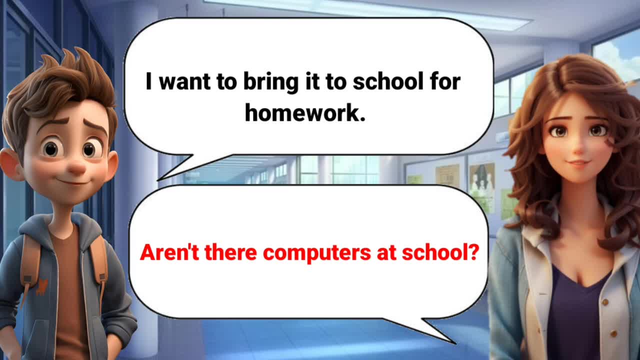 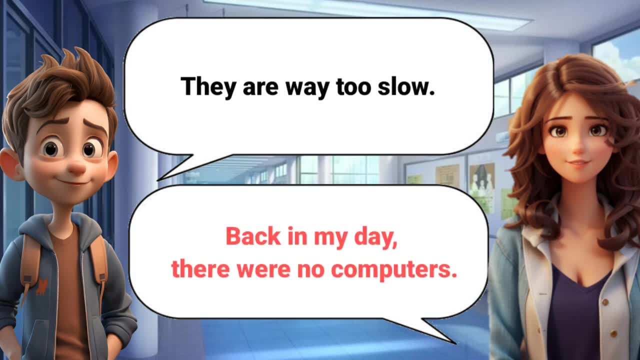 I want to bring it to school for homework. Aren't there computers at school? They are way too slow. Back in my day there were no computers. They are way too slow. Back in my day there were no computers. I hate it when you say that. 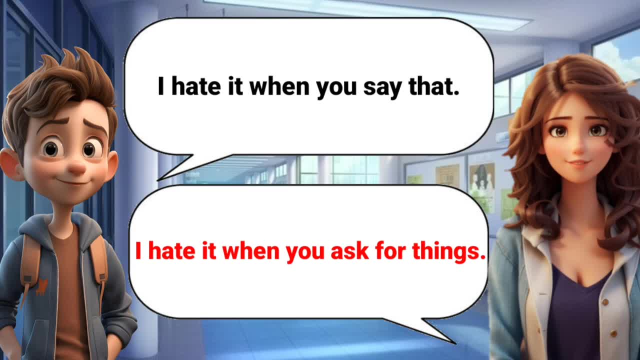 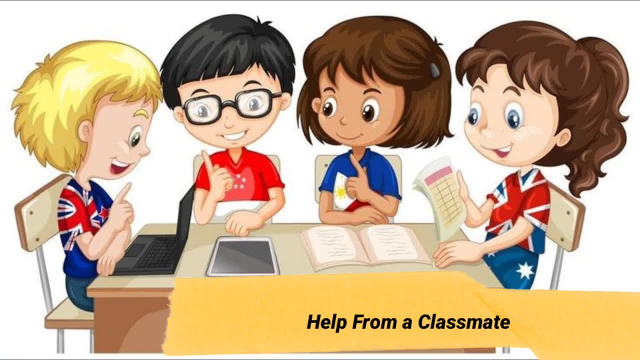 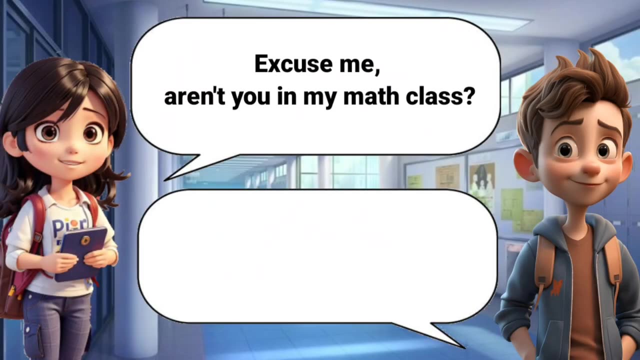 I hate it when you ask for things. I hate it when you say that I hate it when you ask for things. Help from a classmate. Excuse me, aren't you in my math class? Yes, I think I am. 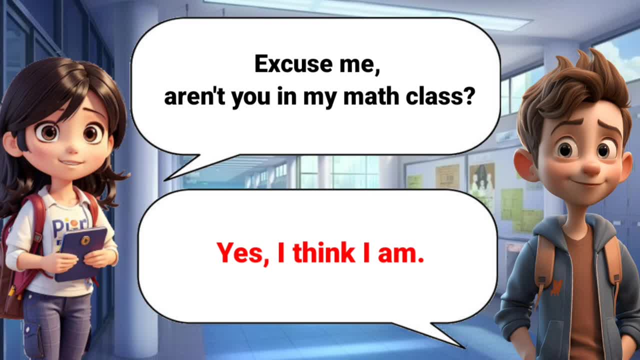 Excuse me, aren't you in my math class? Yes, I think I am. Could I please borrow your notes, Sure, but please hurry with them. Could I please borrow your notes, Sure, but please hurry with them? I will, I only want to look over them. 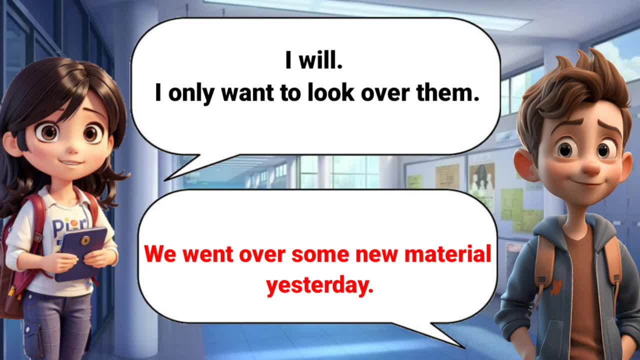 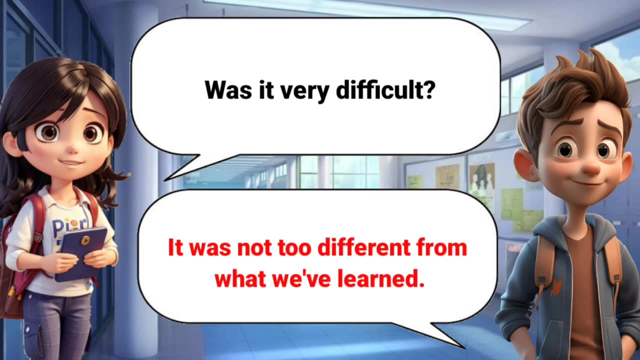 We went over some new material yesterday. I will- I only want to look over them. We went over some new material yesterday. Was it very difficult? It was not too different from what we learned. Was it very difficult? It was not too different from what we learned. 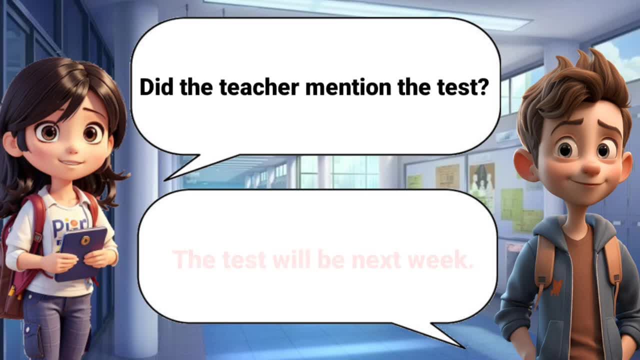 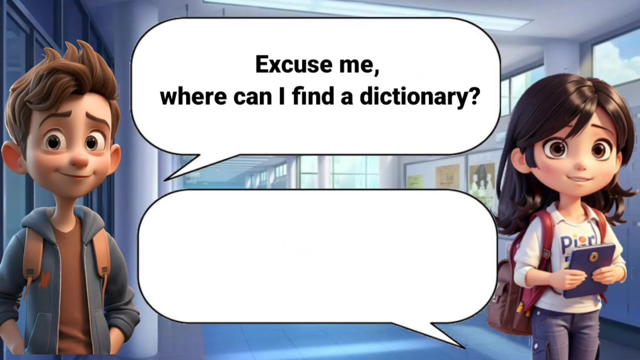 Did the teacher mention the test? The test will be next week. Thank you for your help. Sure, good luck studying English Dictionary. Excuse me, where can I find a dictionary? What kind of dictionary would you like? A bilingual dictionary would be nice. 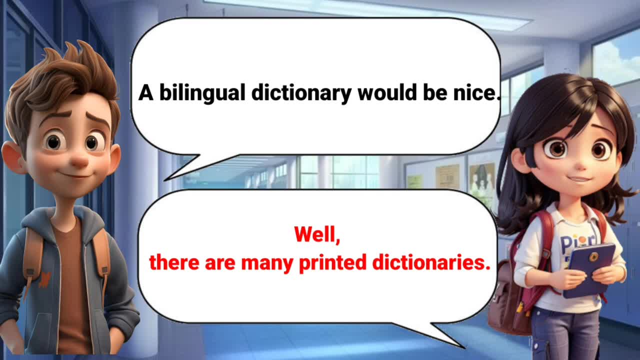 Well, there are many printed dictionaries. A bilingual dictionary would be nice. Well, there are many printed dictionaries. Well, there are many printed dictionaries. Is there one you recommend? Personally, I like digital dictionaries. Is there one you recommend? Personally, I like digital dictionaries. 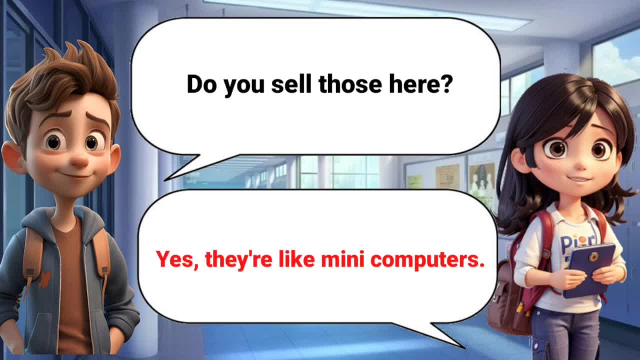 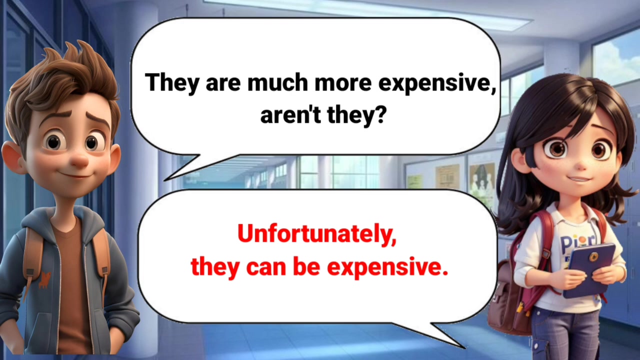 Do you sell those here? Yes, they're like mini computers. Do you sell those here? Yes, they're like mini computers. They are much more expensive, aren't they? Unfortunately, they can be expensive. I think I'll stick with the printed version.